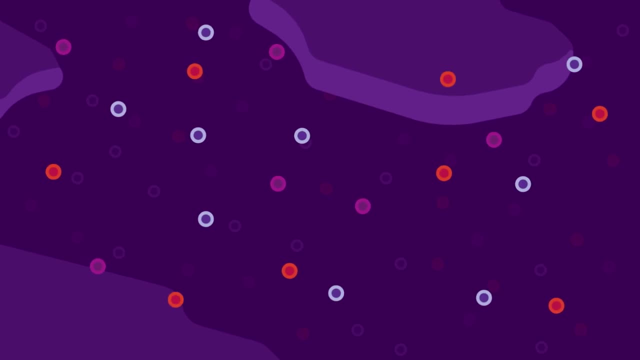 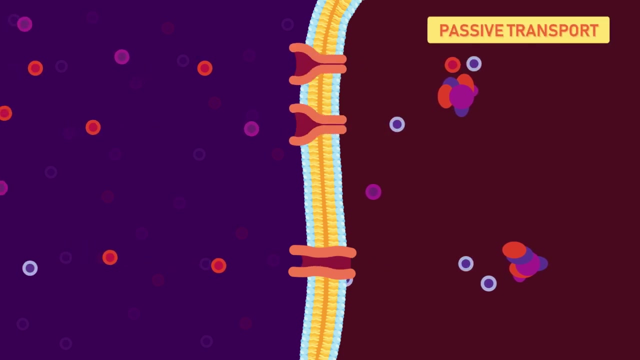 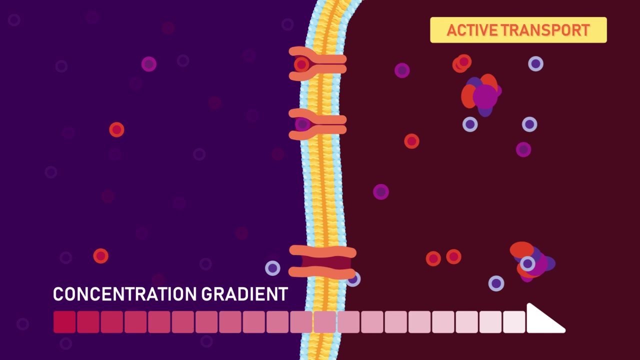 metabolism, Plants take up these mineral nutrients in the form of ions. This uptake of minerals can either be a passive process, termed as passive transport, which takes place along the concentration gradient, thus requiring no energy, or an active process, termed as active transport. 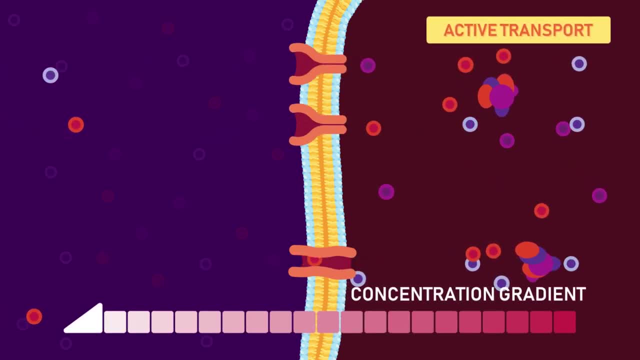 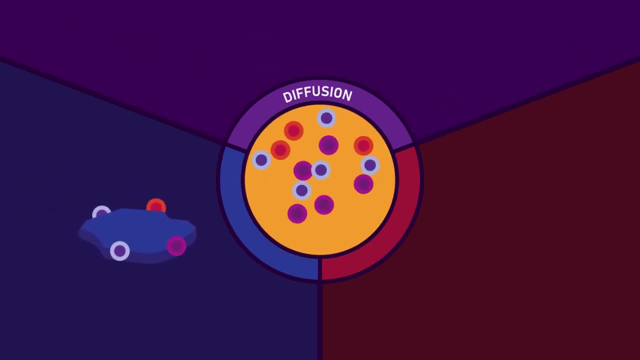 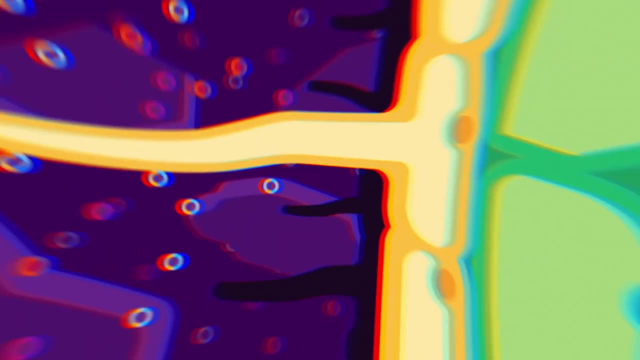 which requires energy because it occurs against the concentration gradient. The passive process- transport or absorption- can be explained by diffusion theory, the ion exchange theory and Donan's equilibrium Diffusion theory. When the concentration of mineral ions is higher in the external soil solution than the root, then the ions in the 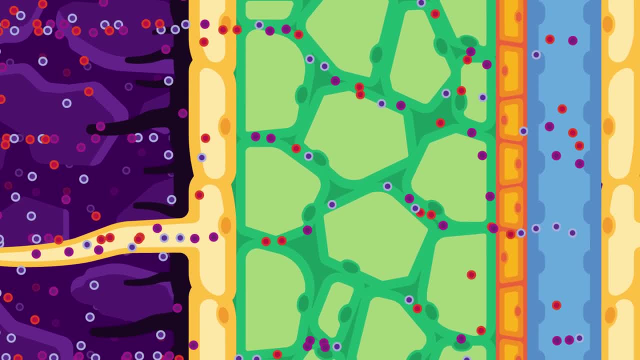 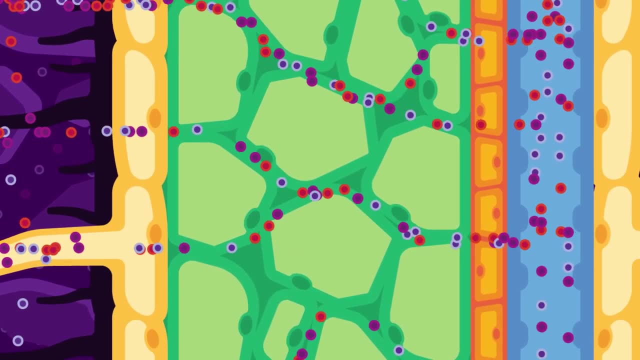 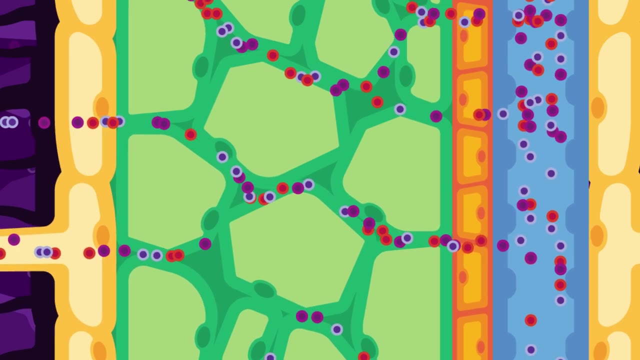 soil solution will move from a region of higher concentration, in this case the soil solution, to a region of lower concentration. that is the roots. This movement of molecules or ions is called diffusion. The ions keep moving inside until an equilibrium is reached. 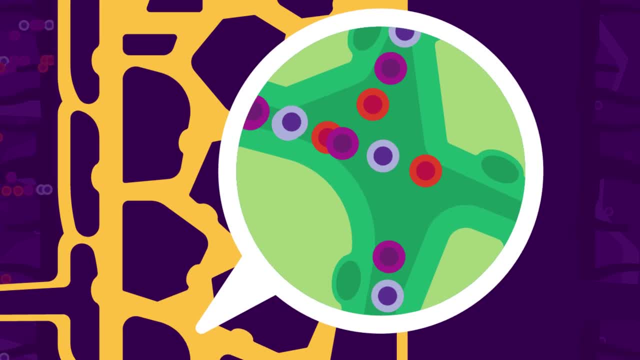 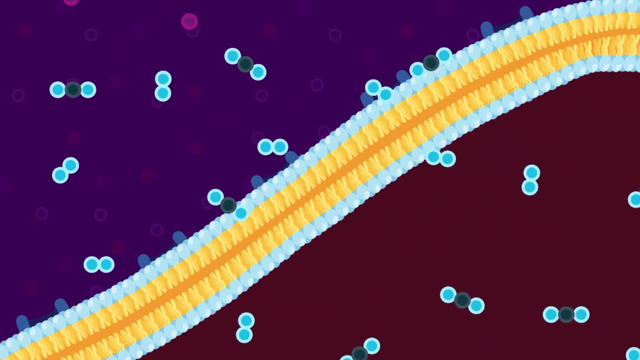 One of the reasons that allows the ions to diffuse into the root cells is because of the apparent free space. However, unlike non-charged molecules, ions will have difficulty to pass through the hydrophilic membrane directly. To facilitate the movement, the proteins 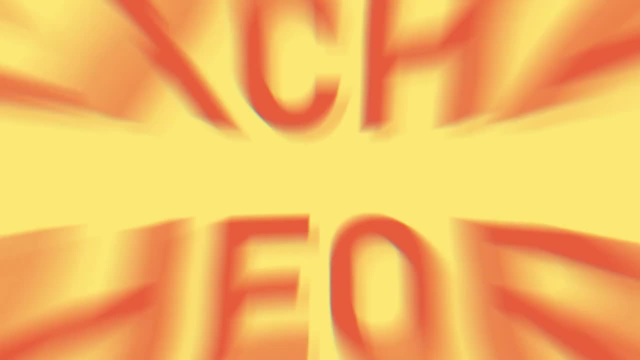 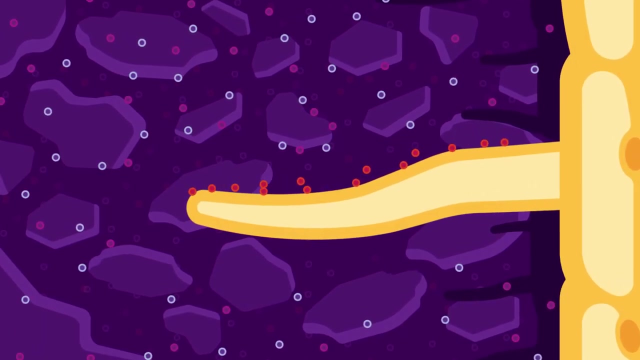 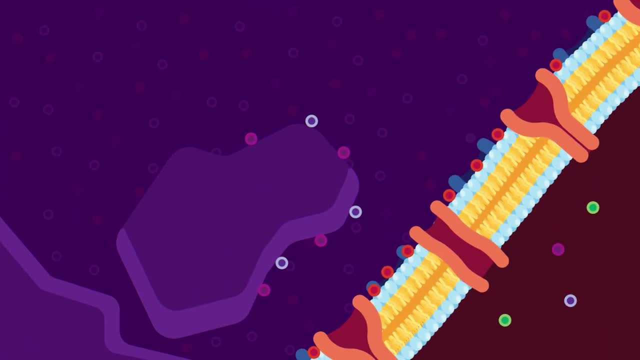 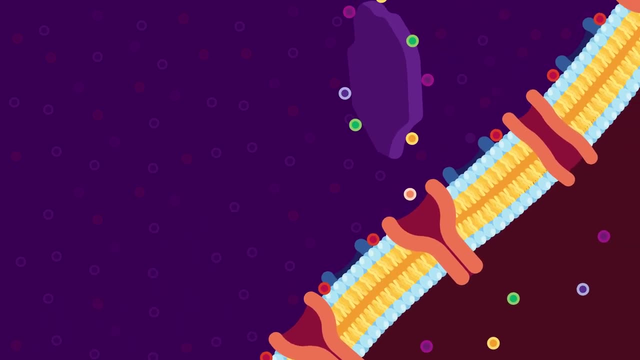 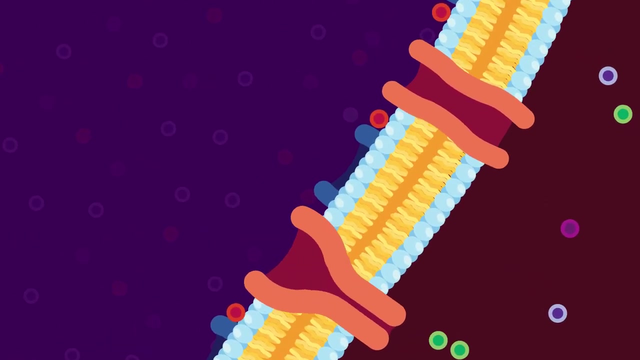 The positively charged hydrogen ions absorbed into the surface of the roots can easily be exchanged with cations of sodium and potassium present in the soil. Similarly, an anion like hydroxyl ion from the root cell can be exchanged with anion present in the soil. Ion exchange can be. 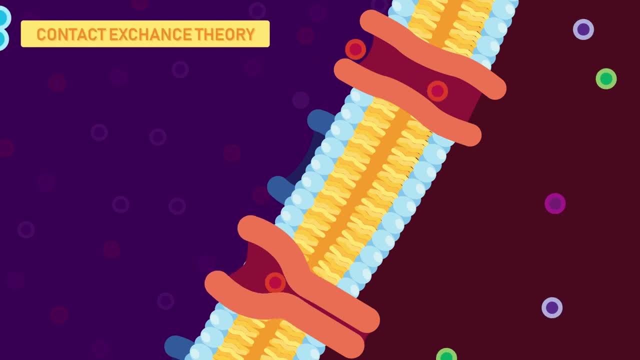 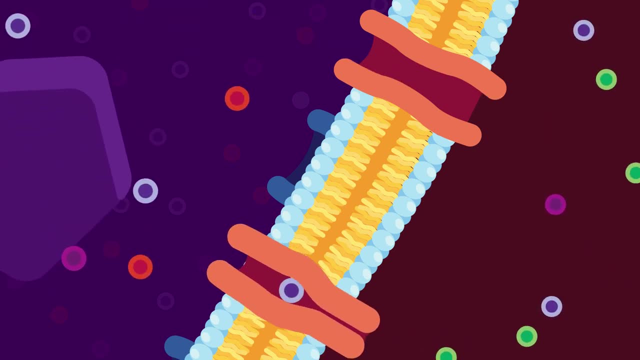